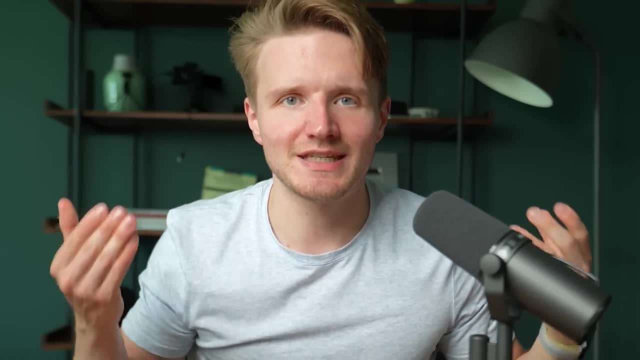 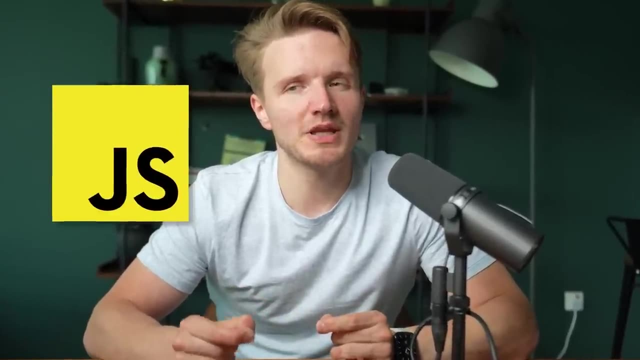 so goddamn difficult to get what you learn to actually stick in your brain and how to fix that. Before we talk about all of that, it's good to understand why exactly is JavaScript such an important language for everyone, So let's get started. 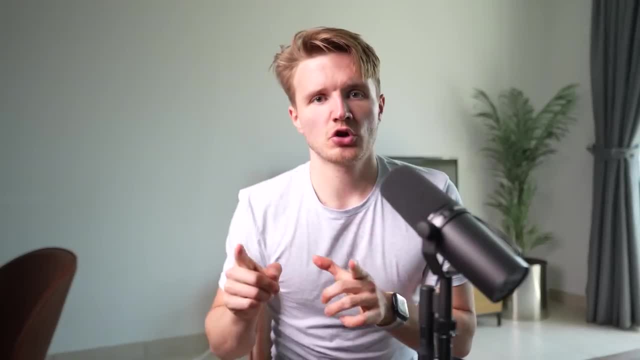 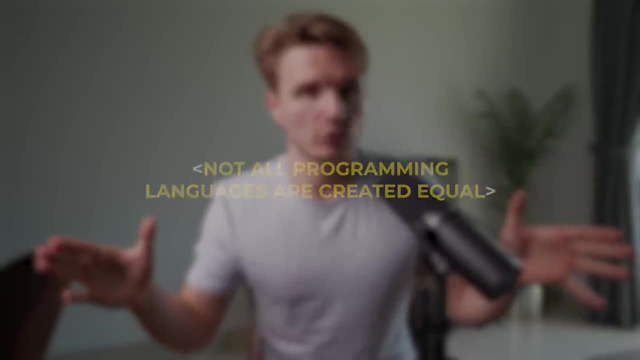 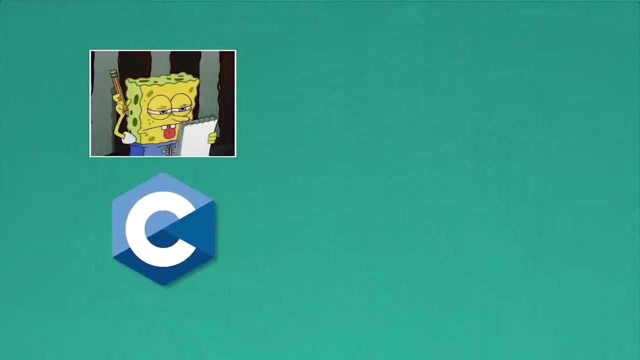 If you're trying to learn to code to get a job, it's useful to realize that not all programming languages are created equal Because, firstly, some of them are much harder to learn than others. If you try to learn something like C, it's going to take you a lot longer than learning something like Python or JavaScript. 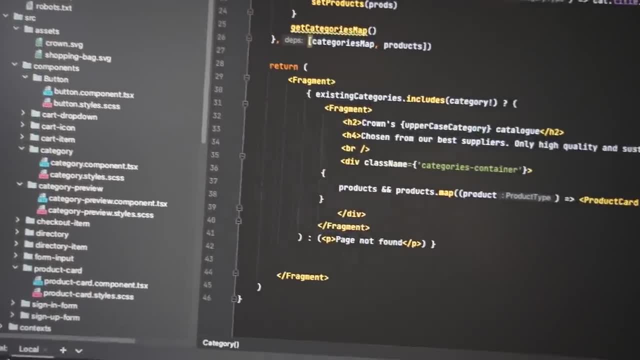 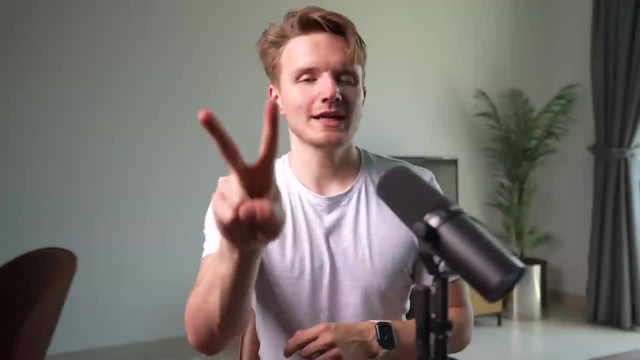 because languages like JavaScript and Python are something that we know as high level languages, meaning that they hide a lot of underlying detail for you to make it easier for you to write code. and the second factor is that some languages are simply in more demand in the industry. 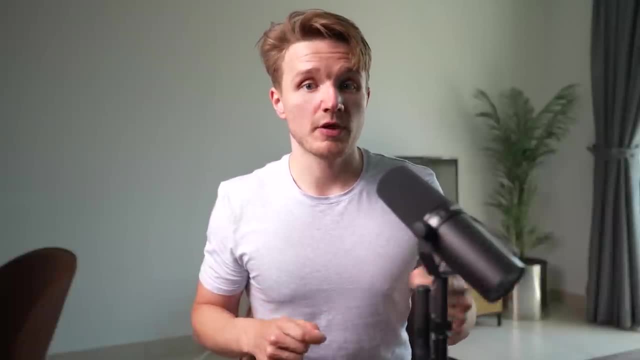 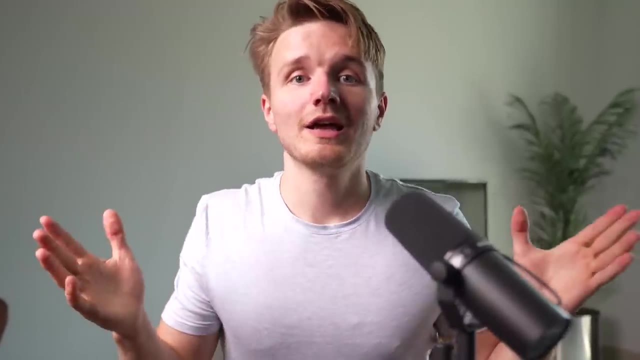 there's more companies using them and therefore more jobs available for them. So ideally, we want to choose the language that's easy to learn And that also, at the same time, has a lot of job demand for it. And luckily, language like that does exist: It's called JavaScript. 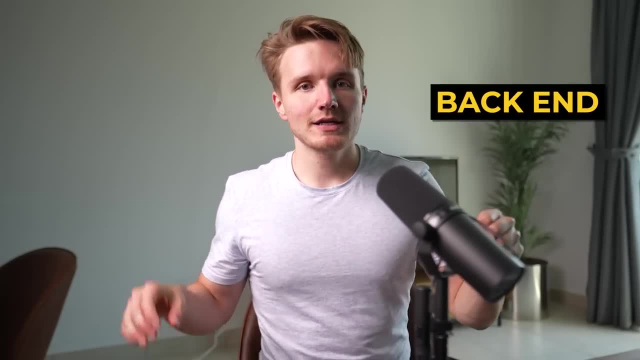 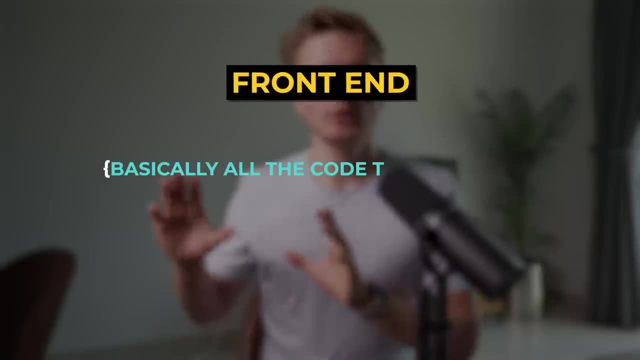 Basically, when you want to build a website or a web app, you have something called a backend and a frontend. The backend can be written in a bunch of different languages, like Python, JavaScript, whereas the frontend, which is basically all the code that 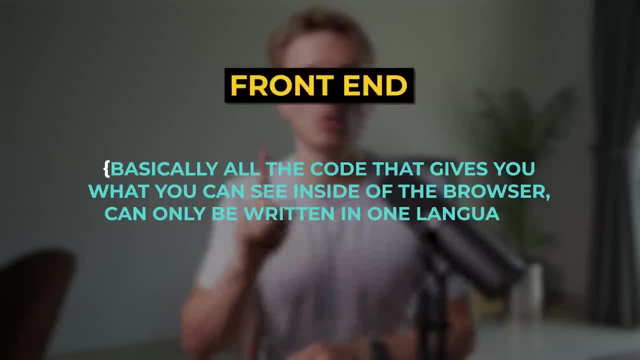 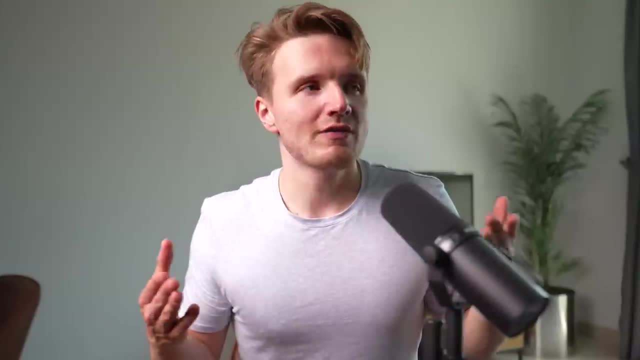 gives you what you can see inside of the browser and only be written in one language: JavaScript. So if you want to get jobs in web development- which is where most of the jobs are, by the way- you don't have a choice. you have to learn JavaScript at some point, And for that reason, 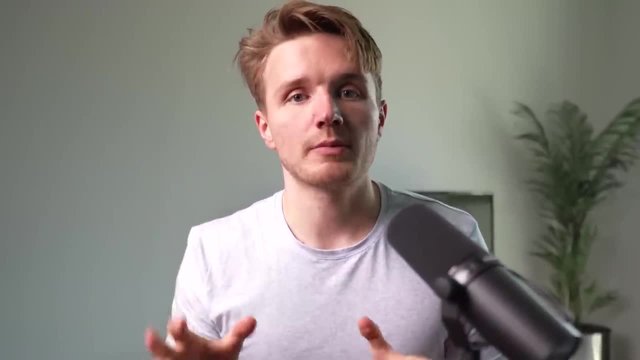 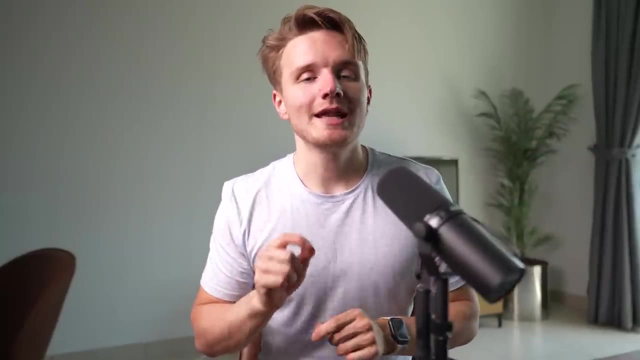 besides Python, it is one of the only two beginner programming languages that I recommend people learn, And I'll get back into the whole debate of Python versus JavaScript, on which one's the big, in a moment, But first let's look at the exact steps that you should take right now to 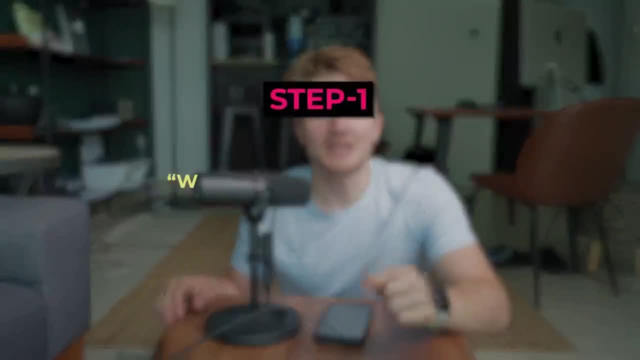 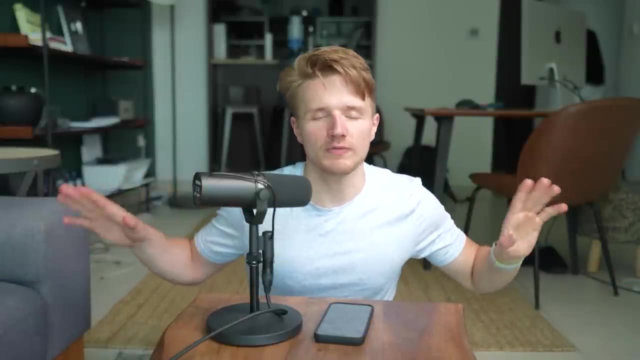 master JavaScript and get hired as fast as possible. Our first step is that, well, we need to get started, don't we? Oh, but which course do I need to do? There's hundreds of possible courses out there, hundreds of tutorials, all of this. 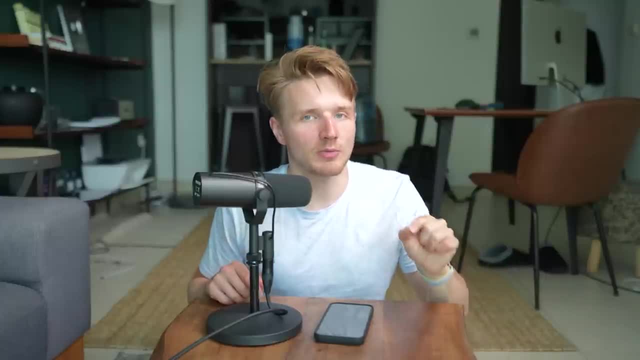 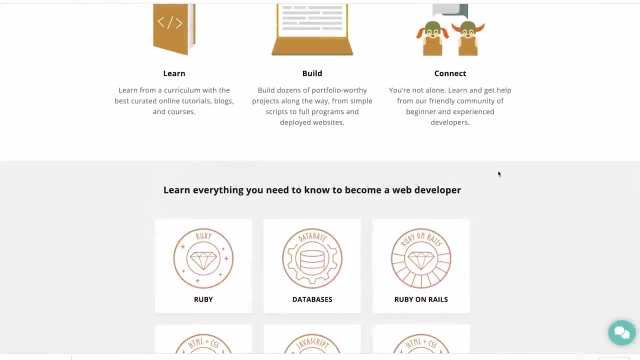 all of them will work, But if you want me to tell you exact recommendations, here are my two favorite ones. The first one is absolutely free and it's called the Odin Project. This is what I personally started with back in the day, because I was broke and I was finding the 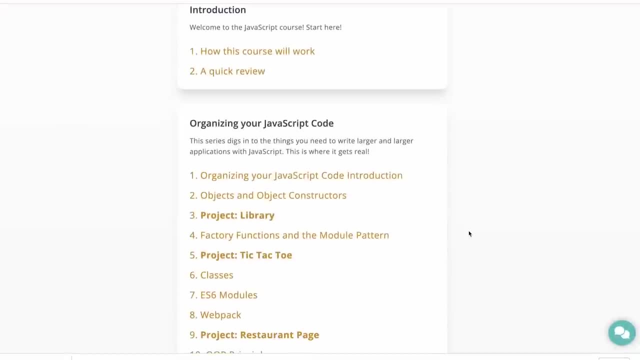 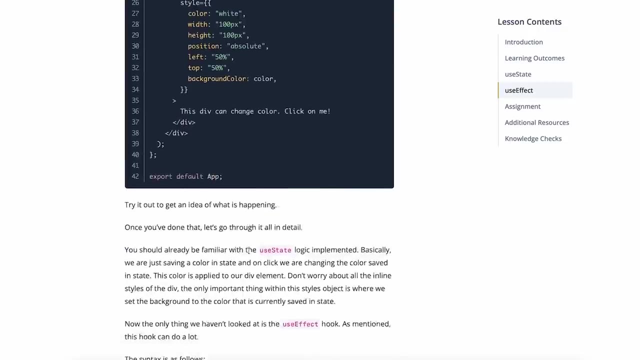 free way to start learning web development At the very least. I recommend you read like the first couple of sections, because the explanations of how the web works and all is really, really excellent. It's just text-based articles, But if you're looking for a free way, 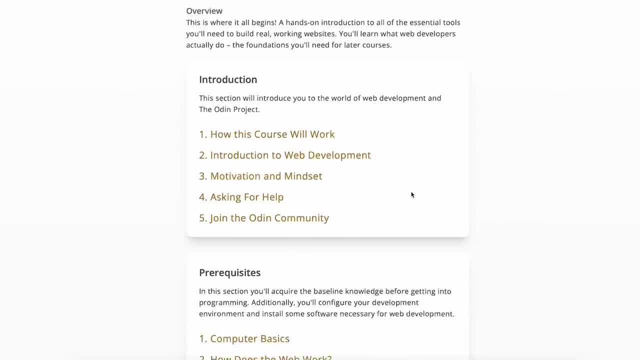 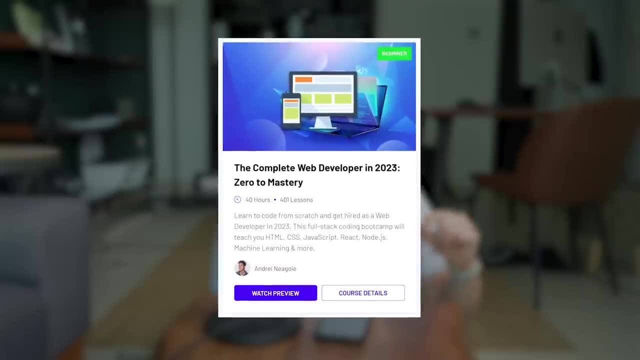 to learn JavaScript. at this stage of your learning, you should go through the foundation sections of the Odin Project, and it's absolutely excellent. The second one, which is my personal favorite, is Zero2Mastery's Web Developer Online Full Bootcamp- Essentially what this is. 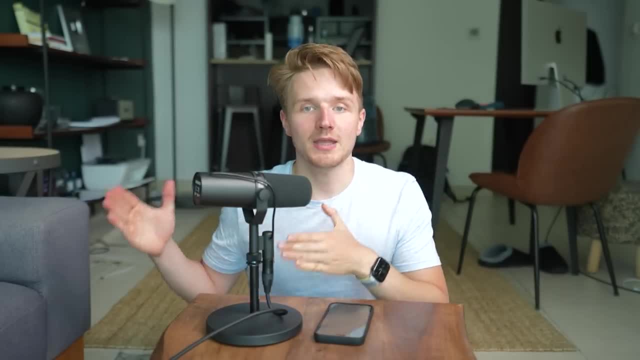 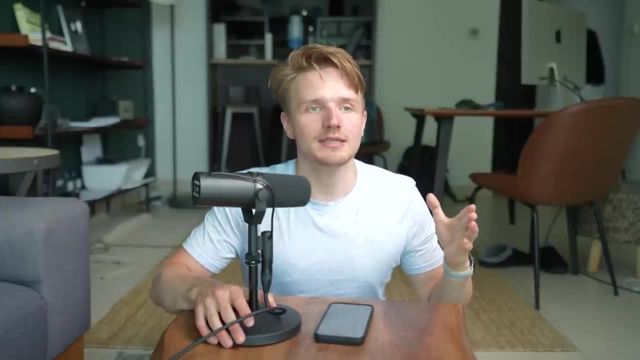 is a full video course, from completely zero to becoming a web developer. It is your JavaScript, HTML, CSS, how the web works, everything that you need, And the thing that I always say is that it doesn't matter what resource you pick, it doesn't matter what course you take, it doesn't. 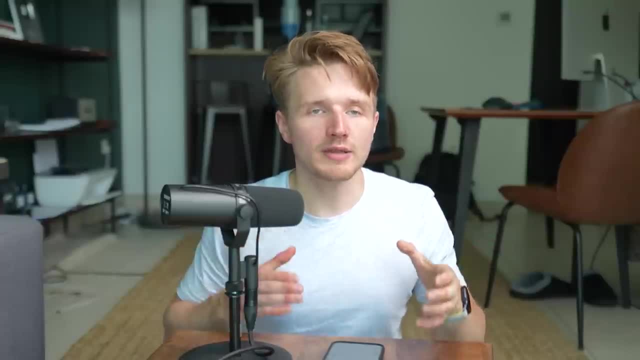 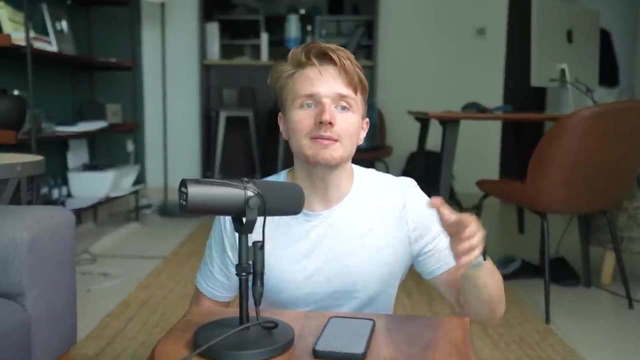 matter what you pick, Just pick something that you resonate with. The best resource is one that you can stick to, And the Zero2Mastery's courses for me are excellent for that precise reason. These are some of the courses that I've used the most in my own journey. They're not sponsoring. 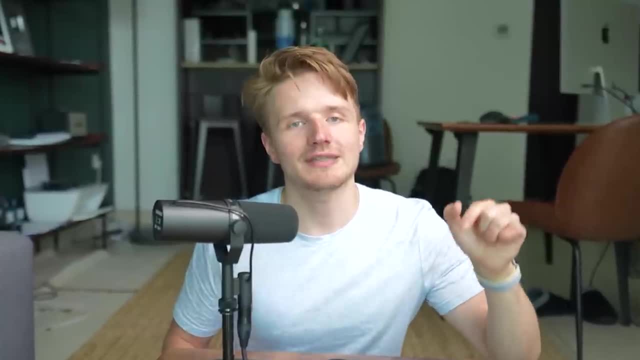 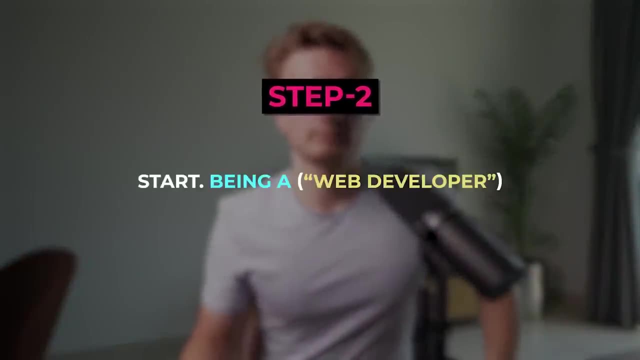 this, but I'm choosing to be affiliated with them for that reason, And I do have a 10% discount code for you down below. Highly recommend you check them out. And the second step is to start being a web developer. That's it, Okay. I think that requires a bit more explanation, right? 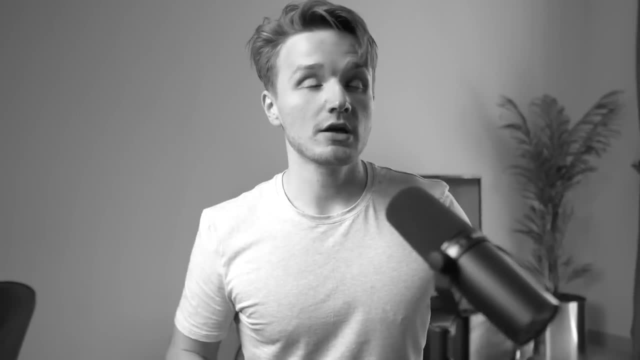 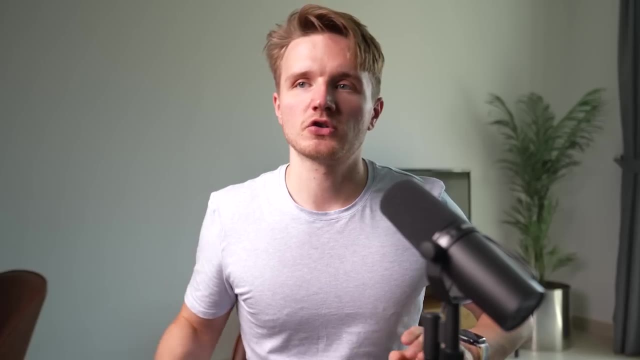 How can I be a web developer if I want to just learn the basics? The thing that most people will tell you is that you need to memorize all of these details. You need to understand async functions, call stacks and all these things before you can start writing. 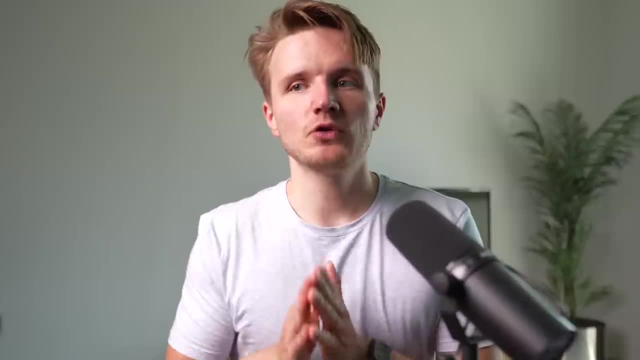 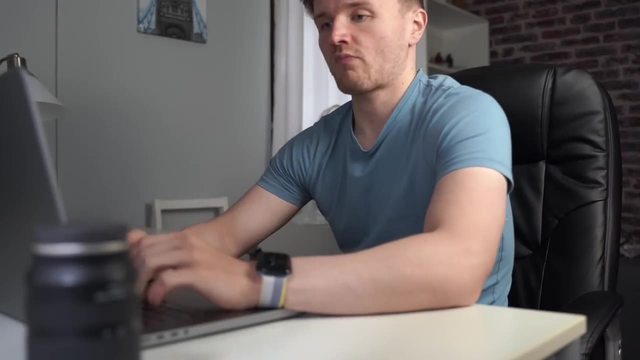 code. But the problem with this kind of learning is that if you try to learn everything before you apply any of it, you will just end up forgetting almost all of it, And then, when it comes to time to actually use it, you're basically still back in square one. 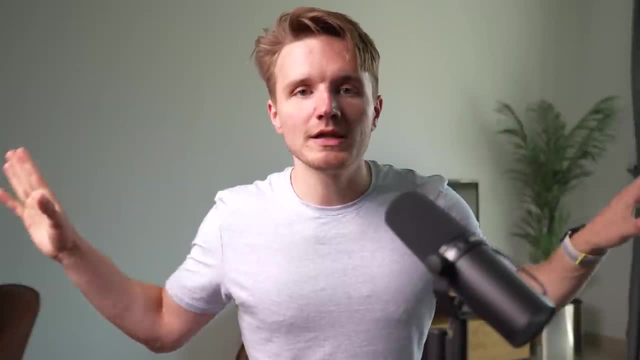 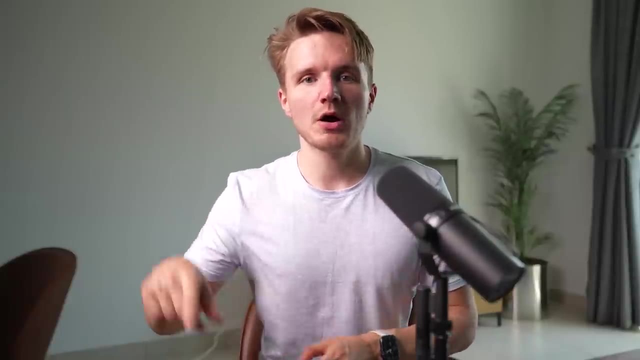 So the philosophy that I used to learn- and this is like my really big thing- is that you should try before you think you can do it. And to really drill this in for you, let me explain this to you by talking about riding a bike. You wouldn't try learning to ride a bike by watching someone else. 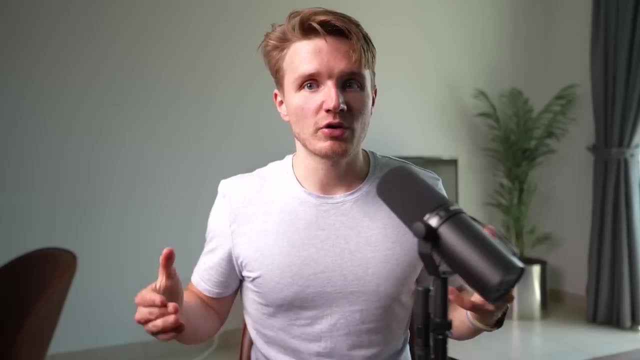 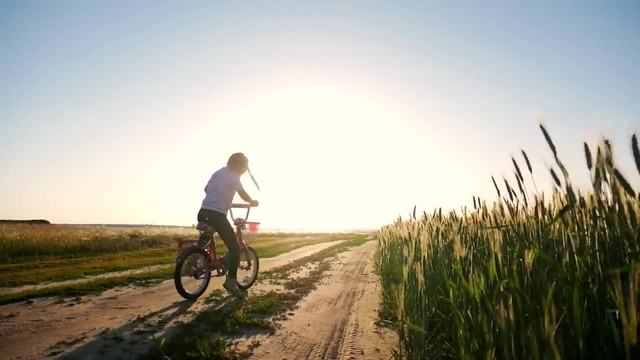 ride a bike. by reading about riding a bike. You would learn to ride a bike by actually riding a bike right And by first riding it really badly and falling a bunch of times. you would eventually get better through trial and error, And this is the uncomfortable process. 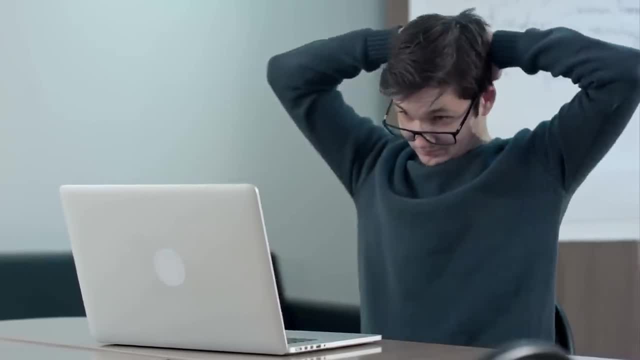 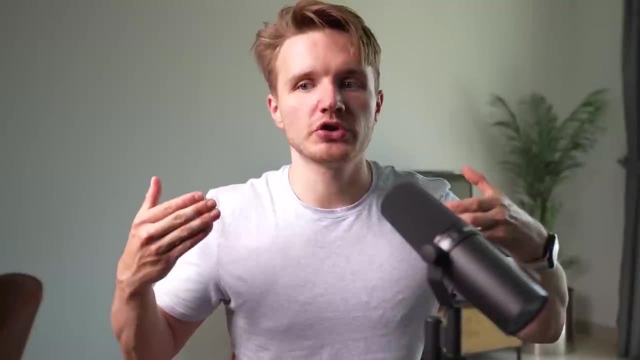 of learning that we all have to go through And all the best programmers go through to actually learn programming skills as well. If you try to give your brain information without context, it's not going to understand that it's important and it's not going to make it stick for. 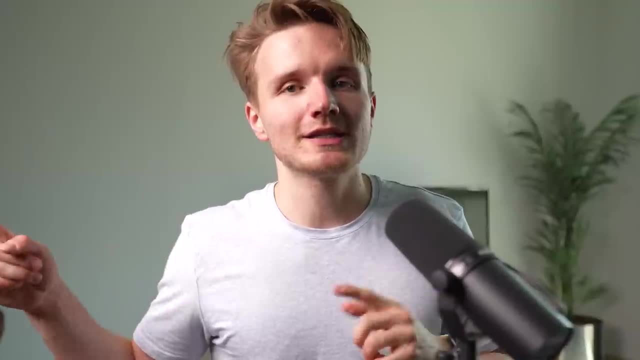 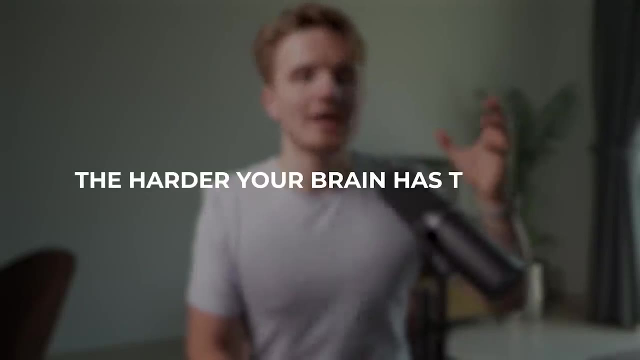 you in your brain. This is why, when you learn a bunch of stuff, you end up forgetting it straight after, because you don't do the work of actually trying to apply it. Basically, what science says about learning is that the harder your brain has to work, the more effective your learning is. 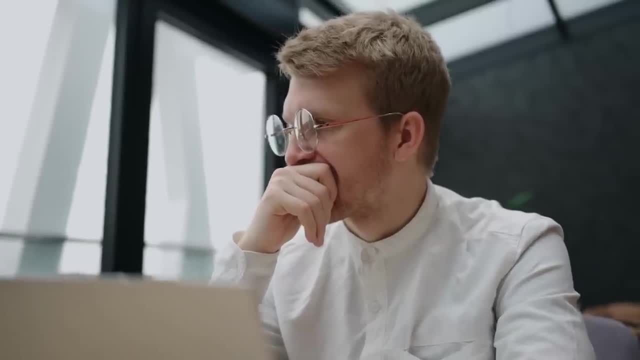 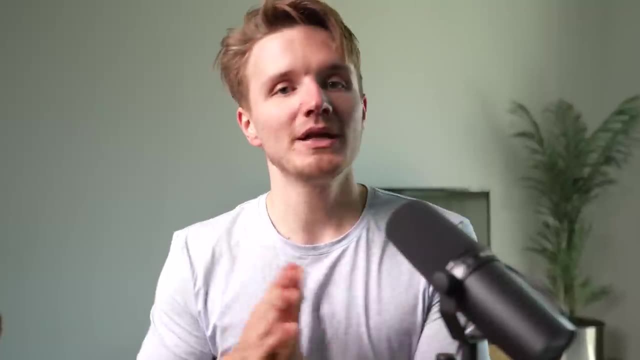 And when your brain is working. the absolute hardest is when you're trying to extract the information out of your brain. You should just pick up a bunch of projects that you don't know how to build yet and then stop building them and figure out the steps along. 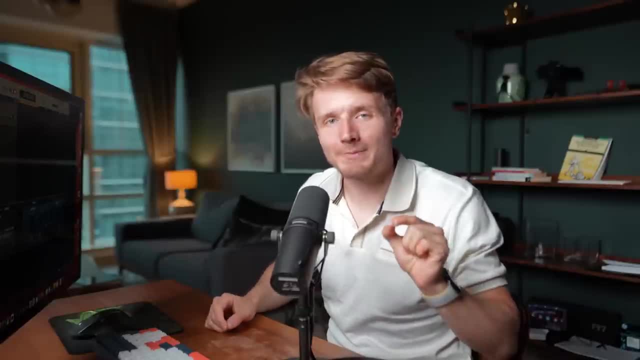 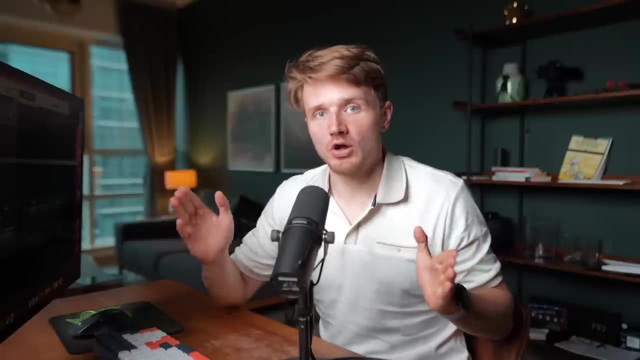 the way. Okay, so at this stage, what we want to be doing is putting in as many reps- as I like to call them- as possible when it comes to just coding a lot of JavaScript, Because the thing is, the more you code, the more you learn. The best tip that I can give you when it comes to, like how to actually 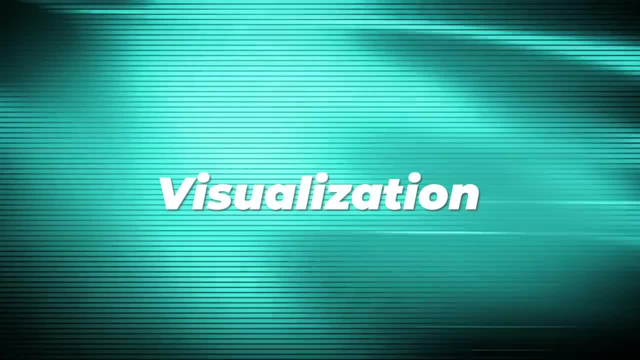 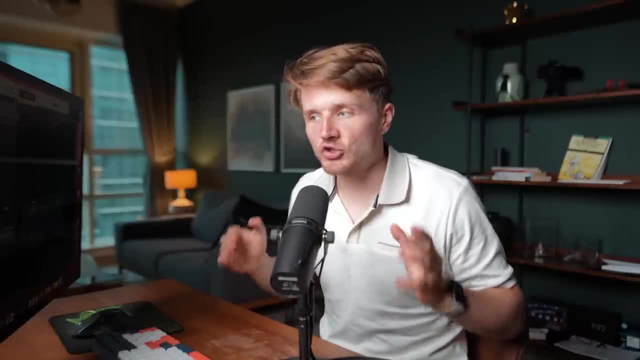 learn really fast is using a technique called visualization. For me, when I can see the output of my code in front of me, it makes it so much easier for me to understand. It allows me to learn what I want to do. And the issue is, with a lot of IDEs it's sort of difficult to visualize. So 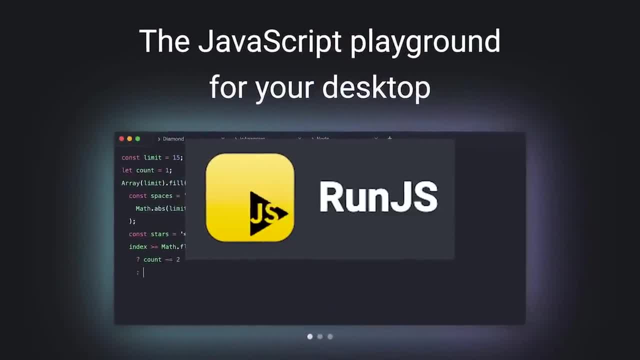 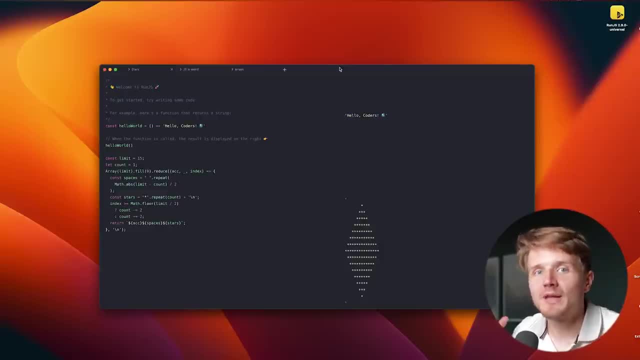 that is why what I recommend you do is download this tool called RunJS. What this is is essentially this minimalist window that you can have open to instantly visualize your code, And this is like absolutely amazing, And I wish I had this when I was starting out, For example. let's say: right, 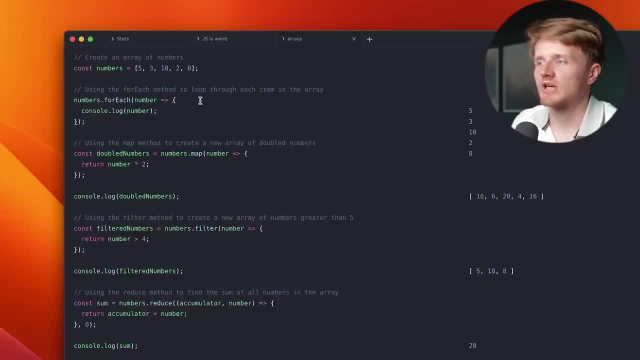 here we're practicing array method, So we go down for each and then we want to see, like, what's actually happening, So we console log it. But instead of having to run the code separately, you can just see the result of your code on the screen. 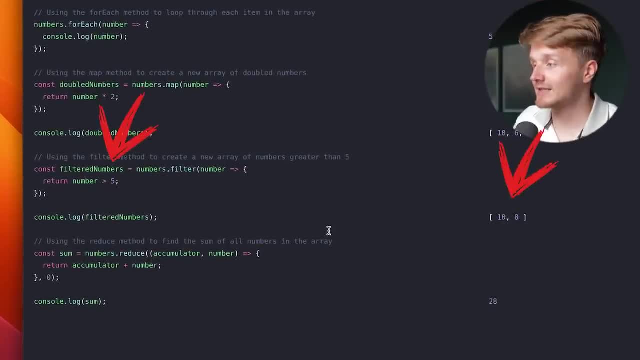 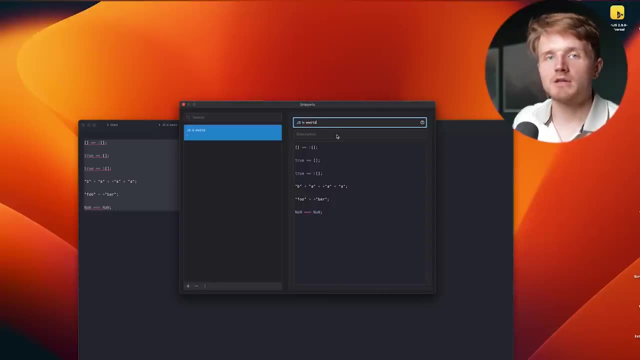 On the right hand side here, and then, when you change things, we can instantly see what's happening. right here You can even test NPM packages without actually having to install them on your computer, And then you can even start building your own code snippet library. 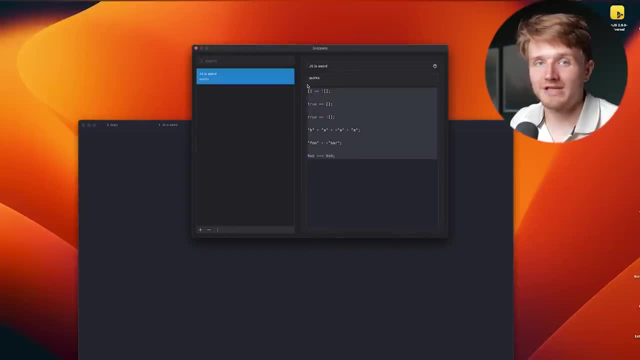 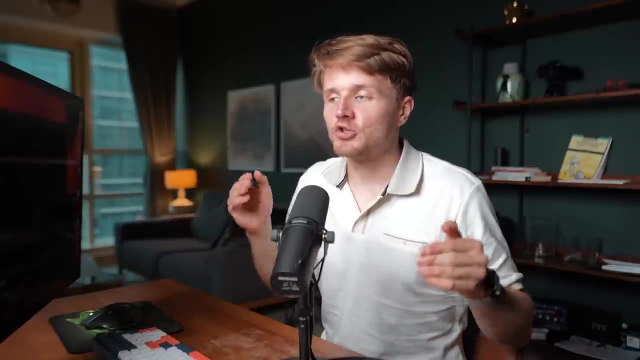 of these pieces of code that you have written to use in other projects as well. This is something that I think is totally revolutionary and something that absolutely every JavaScript developer should be using. So right now, go and download this and have this open with you. 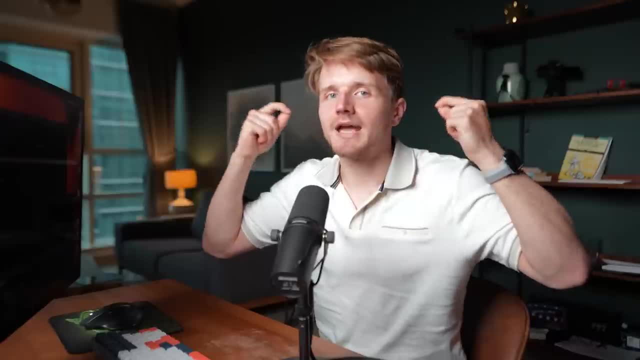 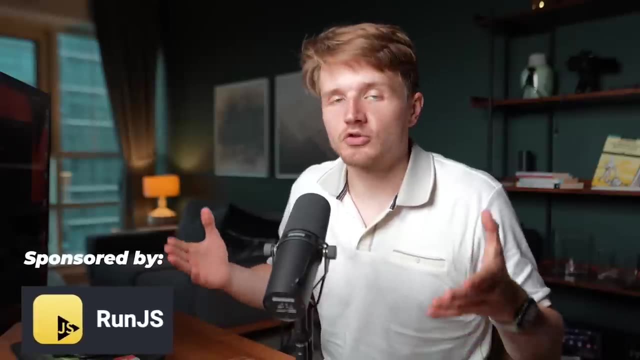 whenever you're coding, Play around with it. This is what's going to start building up that intuition inside of your brain and allow you to start mastering JavaScript really fast. They did sponsor this video, So thank you so much for RunJS for reaching out. This is one. 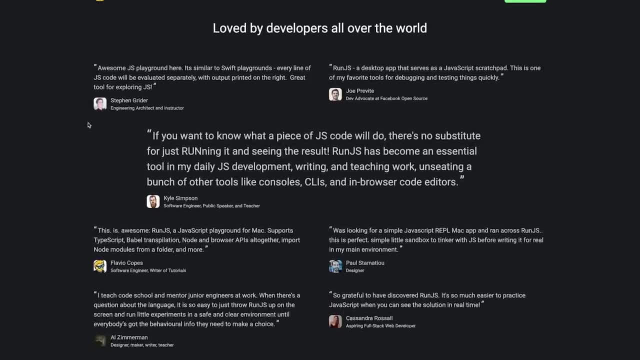 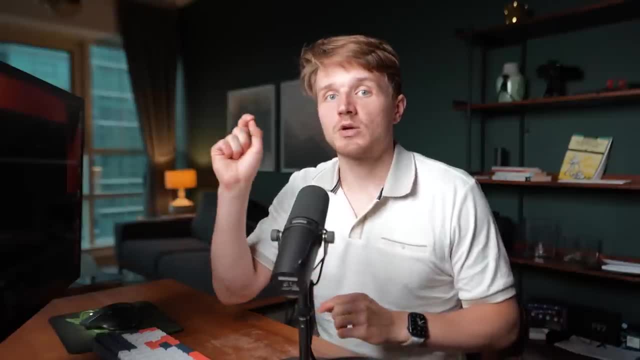 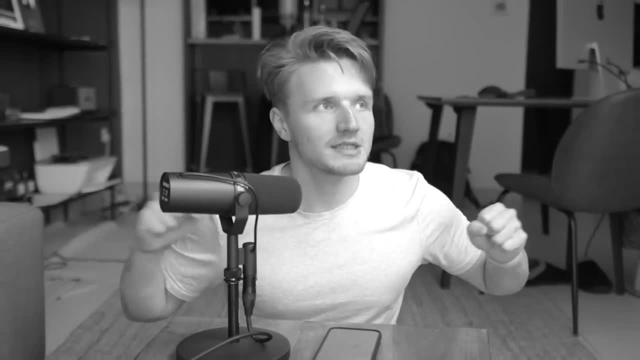 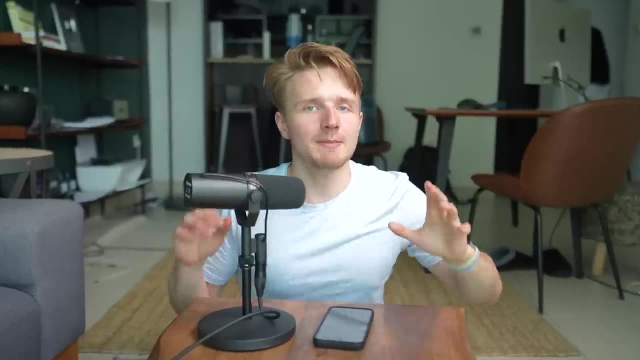 ah, Thomas, I built like five projects using JavaScript. Why am I still not getting interviews? Well, because your projects suck at this point. Okay, The thing is that up until this point, we've been learning basically plain JavaScript with plain HTML and CSS, But the 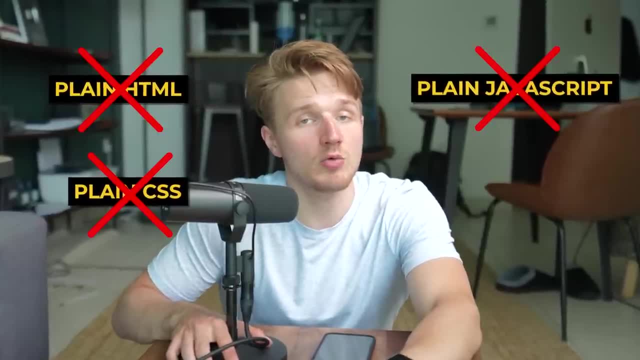 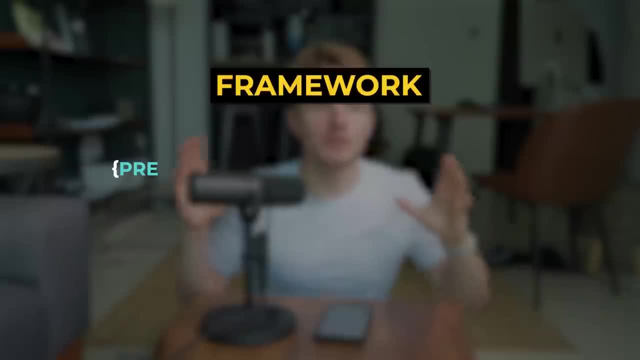 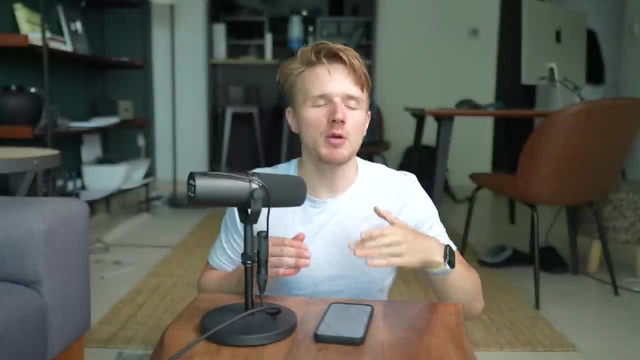 thing is- and I'm sorry to have to tell you this, but in 2023, no one uses plain JavaScript. Everyone uses what we know as framework. What a framework is is basically like a pre-built thing that is built around plain JavaScript to make web development easier for you Remember. 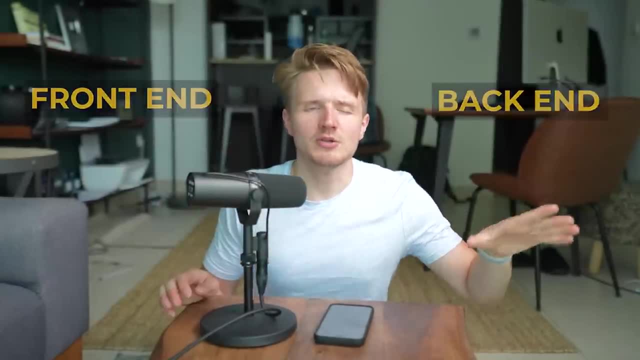 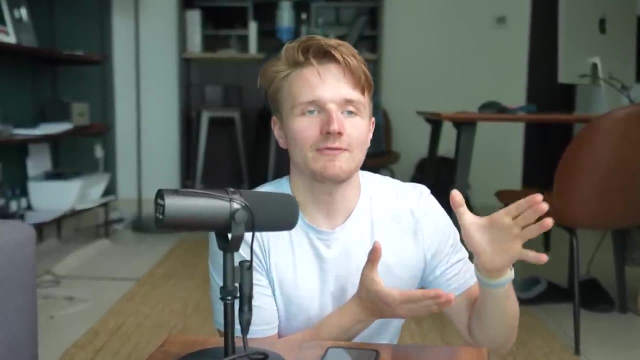 from our explanation before we've got the backend and we've got the frontend, Actually building our server and everything like that manually is pretty complicated. So they've built these pre-built frameworks with everything that you need to start using a server right away. 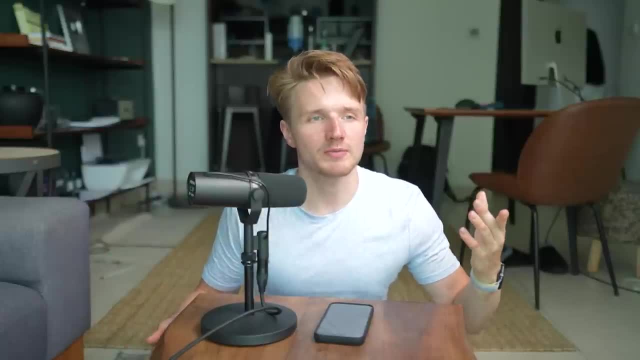 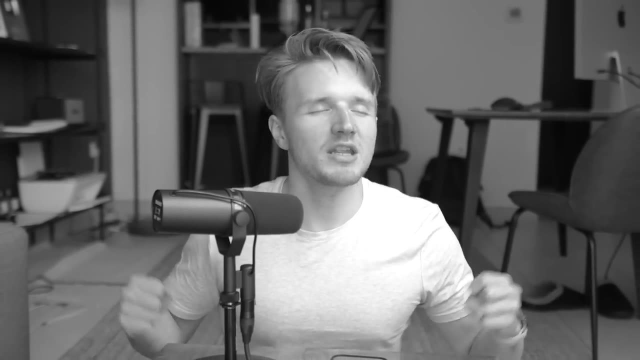 The same thing for the frontend. actually, building out a complex frontend for our website is actually quite complicated, So they've built these frameworks to make it easier for you. But, Thomas, you spent so much time learning plain JavaScript and HTML. if no one uses them, 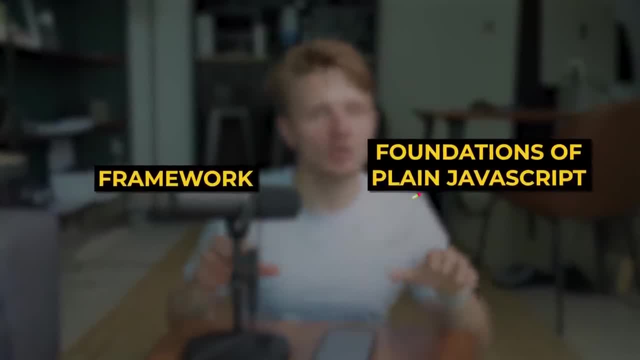 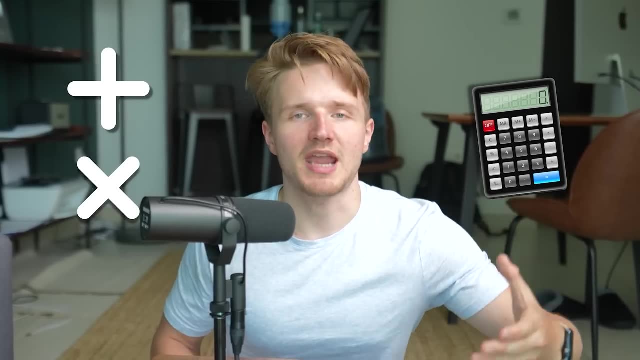 Well, it's because, in order to understand these frameworks, you need to learn the foundations of plain JavaScript first. It's sort of like trying to use a calculator before learning foundations of how additional multiplication works. before that You need to understand the foundations. so 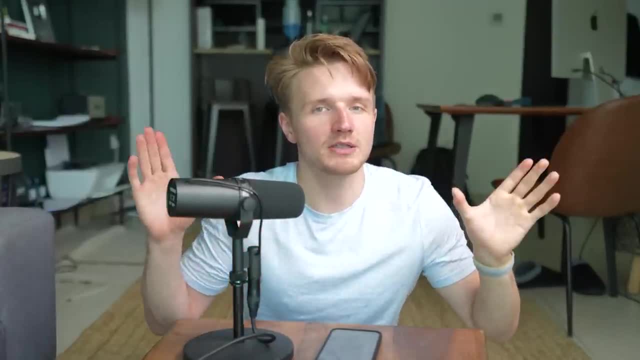 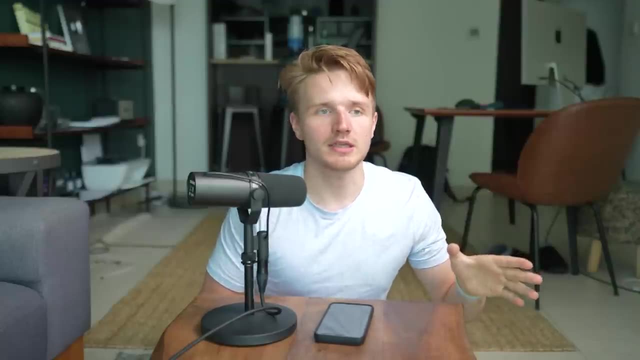 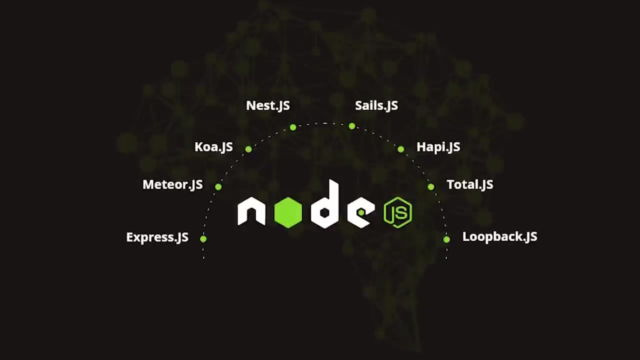 that, then you can essentially ignore them and just start building on top of them. I mentioned before that you can use the backend in many different languages, like Python or Java and things like, But if you've learned JavaScript already, it makes sense for you to also do the backend in JavaScript using this framework called Nodejs and Express. 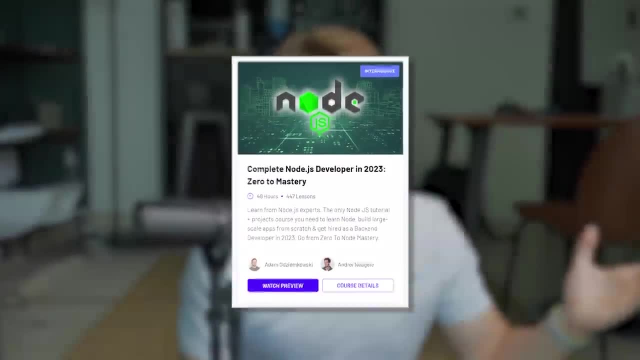 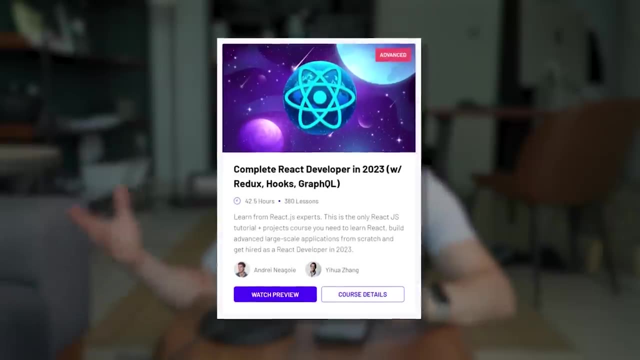 There's a great course again by Zero to Mastery that goes over all of this, including in a very detailed way how the backend actually works, how these frameworks are actually built. If you're more interested in the frontend, Zero to Mastery's React Bootcamp is again absolutely the best choice for me. 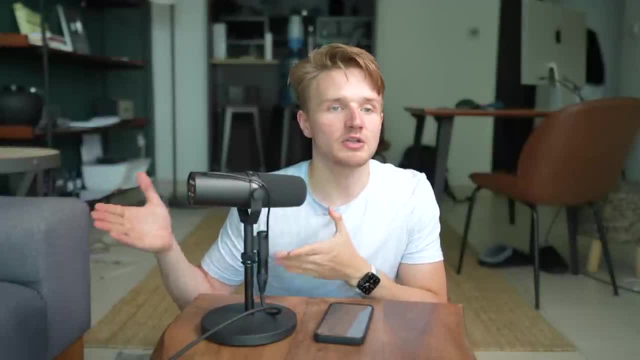 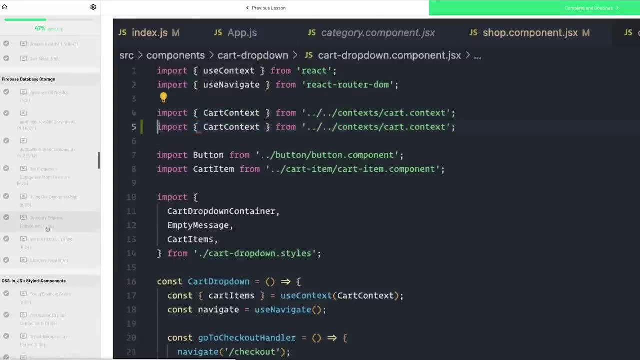 Their React course is honestly probably one of the best programming courses I've ever done, because the way they do it is by essentially building a project as you're going along the course. So basically, at the end of the course you're going to have a really great frontend portfolio project to just put in your resume. 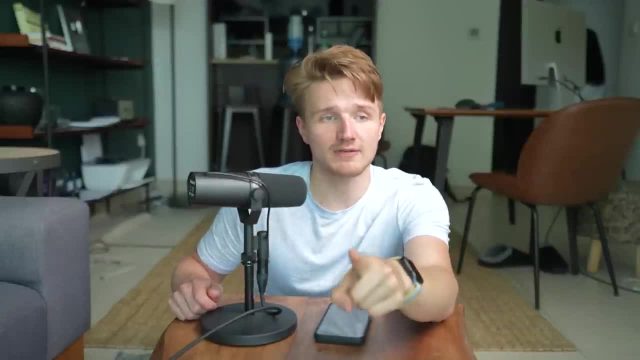 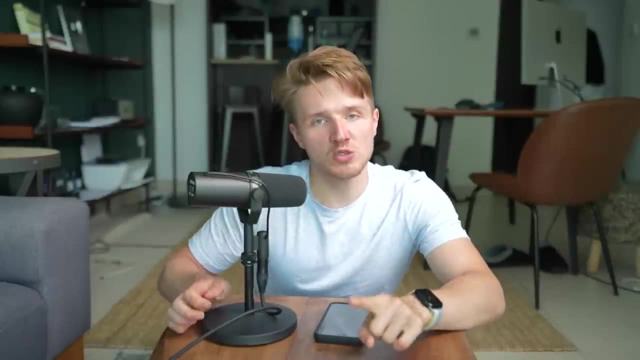 And if you want to be really serious and you want to become a full stack developer, then you want to learn both of these. You want the backend and the frontend. Papa Thomas, how do I know which one I should pick If you don't know which one to pick and you want to pick one of them? pick React. 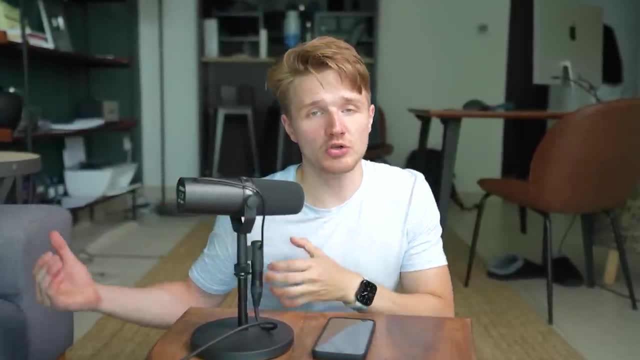 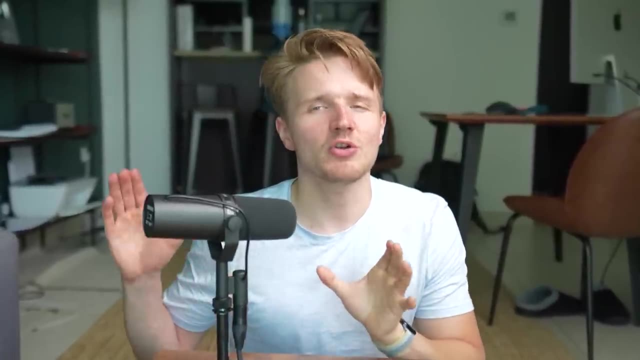 Because the thing is, if you want to get hired, You need to be able to build portfolio projects to show that you know how to code. And it's sort of difficult to build a project just with the backend, without the frontend, So you're sort of going to have to have a frontend anyway. 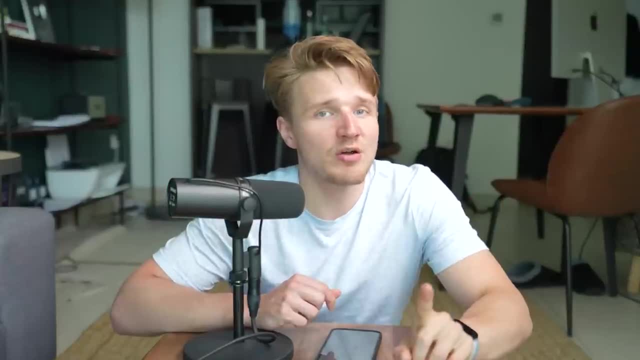 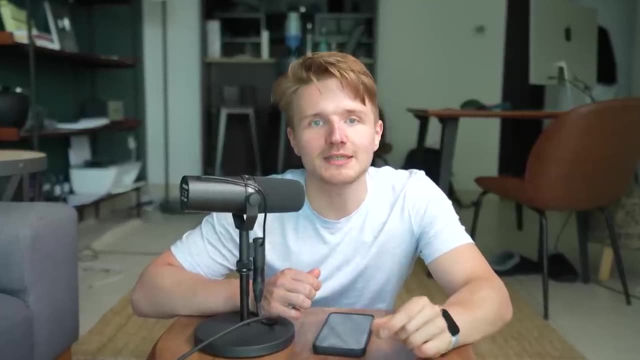 So it makes sense to at least learn the frontend. So now, are you finally ready to start applying for jobs? No, because there's still a massively important step. Unfortunately, 95% of people ignore, which is the reason why 95% of people never get hired. 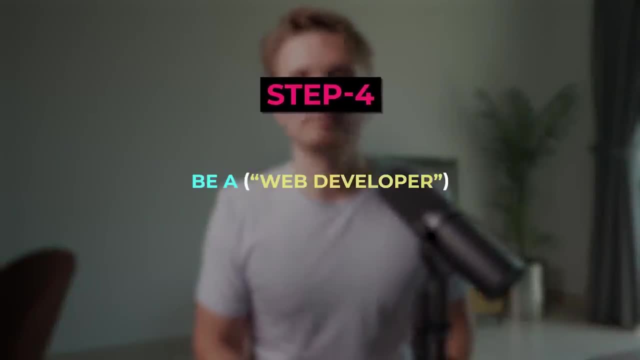 So listen very carefully. Step number four Is to be a web developer again. This time we're coding something serious, And the mistake that you want to avoid at this step is getting stuck on a building stuff that's comfortable for you. Again, remembering: how do we learn. 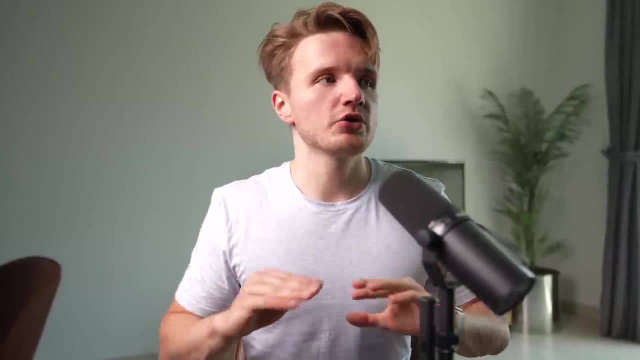 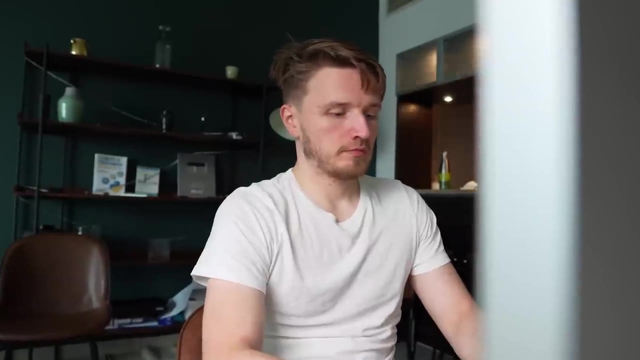 We learn about being uncomfortable. So you need to exit out of building your simple to do apps and weather apps and whatever that we'll find in step two. But now these should be too easy for you And if you keep building these things that are too easy for you, you won't progress and you won't progress to the next level. 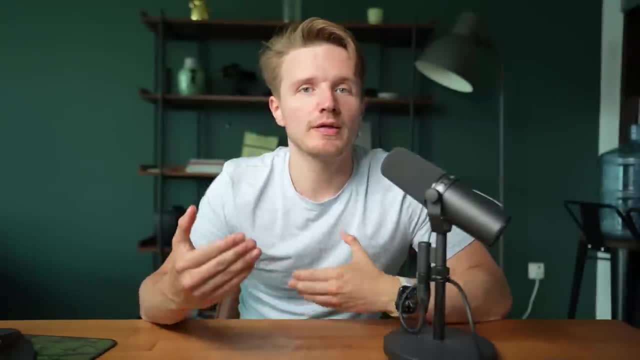 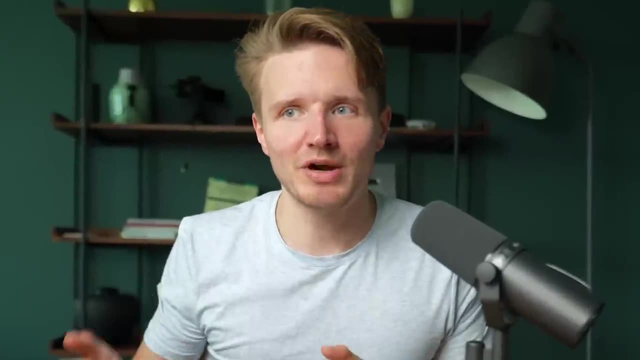 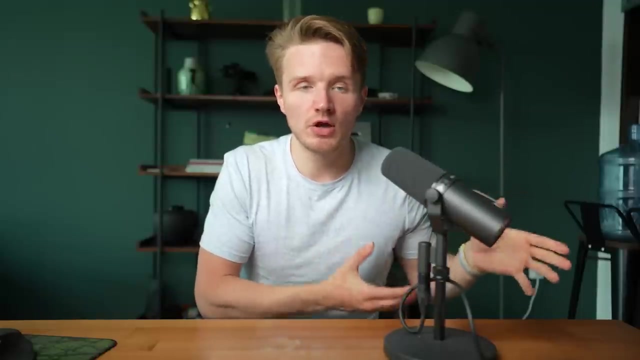 The level of being an actual developer. I hate to break it to you, But the competition for programming jobs is really tough, So that means that this time you do actually need to build something impressive. You need to build something that actually shows that you know how to write code using the foundations of the skills that you've learned this far. 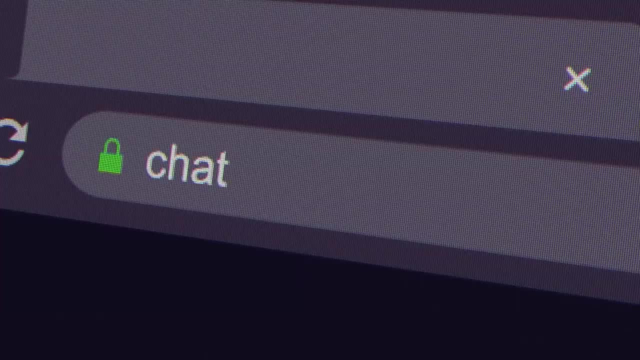 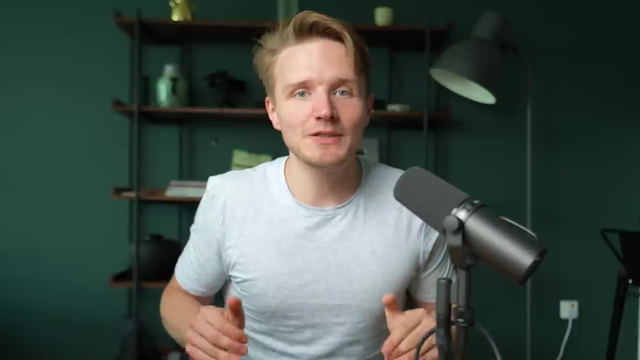 And, quite frankly, just a lot of Googling and using things like chat to aid you again. If that idea scares you, welcome to the tech industry. Like the competition is tough, This is not easy, but you have to put in the work but to hopefully make this like less scary for you.